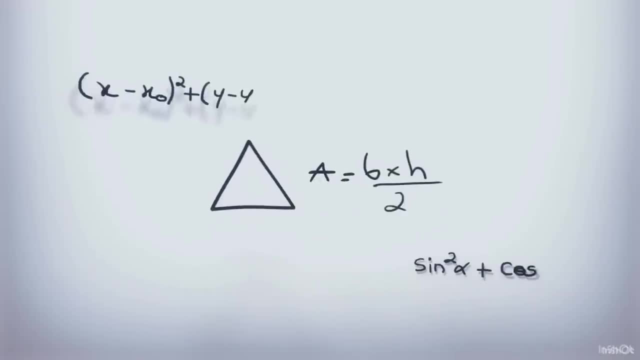 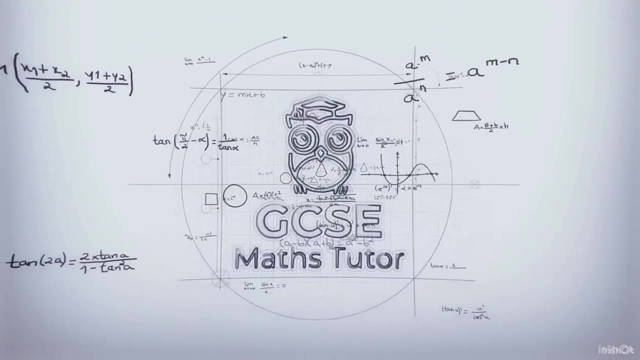 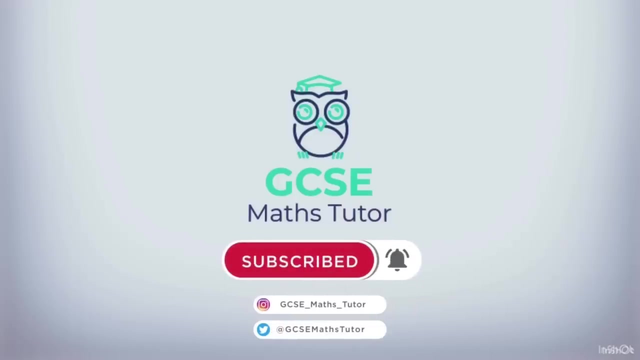 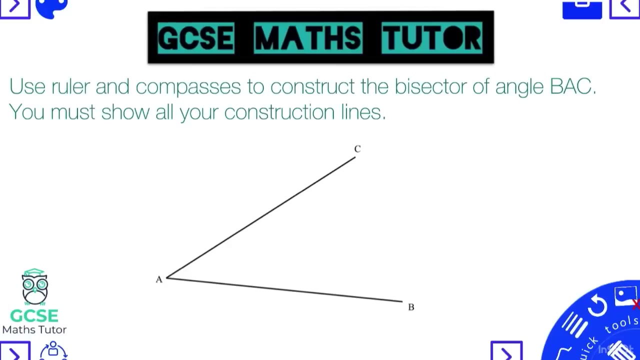 Okay. so in this video, we're going to have a look at angle bisectors and perpendicular bisectors. So for this video, you're going to need some paper, you're going to need a ruler, you're going to need a compass and you're going to need a pencil. We should be. 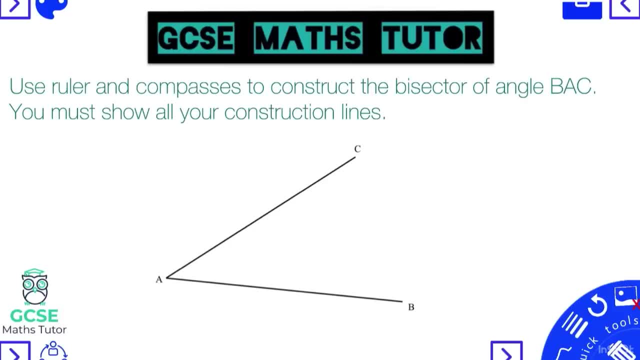 able to do all of those using those bits of equipment. So to follow along with this first one, you just need to draw yourself an angle like the one that's on the screen, around about the same sort of size as the one that you can see, just so that we can actually 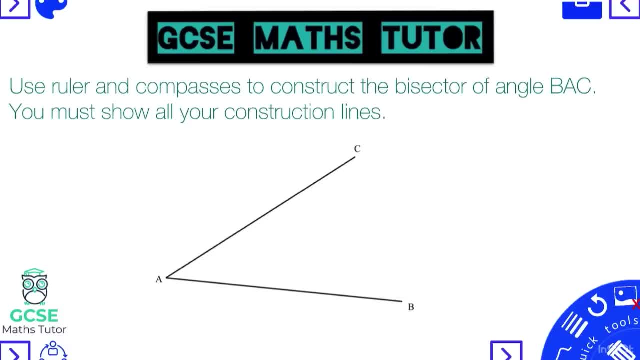 practice going along with this. So the word bisector means to cut in half. So what we're going to do here is we're actually going to cut this angle in half. In other words, we could find out the area between these lines that's closer to the line AC or closer to 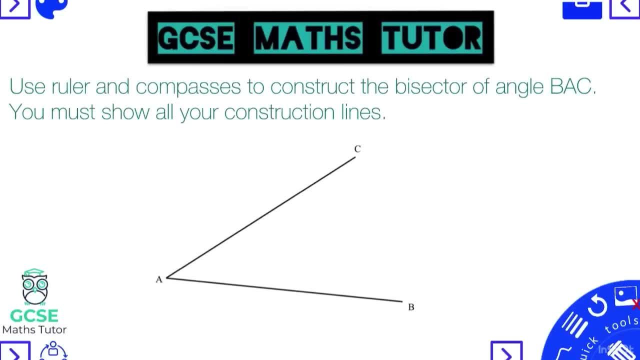 the line AB, And sometimes you might be asked to do that instead, maybe to shade a region that's closer to the line AC rather than AB. Now, for the purpose of this, there are two different ways of bisecting an angle. I'm going to do it one particular way that I just 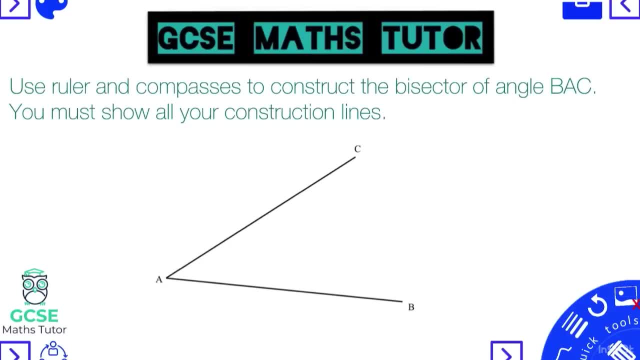 tend to prefer, but there are two different ways of doing this and probably other ways that people have found that they might have seen before, But I'm going to do it one specific way that I think is the easiest. So, first of all, you need to grab your compass, Obviously. 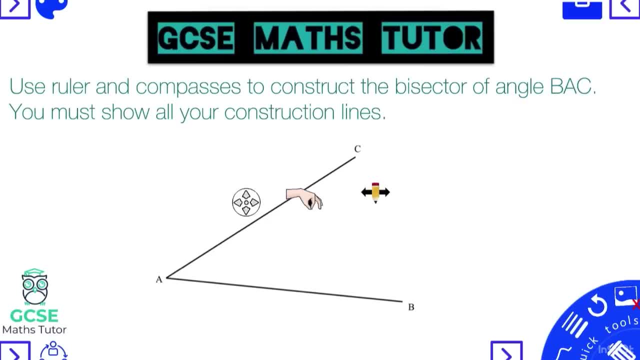 as I'm doing this on screen, it looks a little bit different to a normal compass, but where these arrows are, this is the sharp point of my compass. So what we're going to do is we're going to put the sharp point of the compass right down there where the two 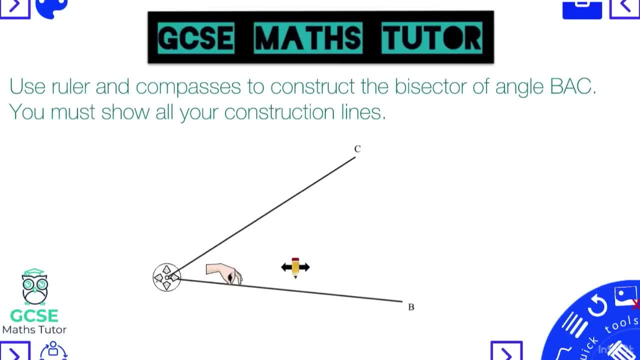 lines meet on the point A, Then what you're going to do is you're going to extend your compass. I'm going to do this in red So you can extend your compass, obviously, with where the pencil is any sort of length. I'm going to go about halfway down. I'm going to do 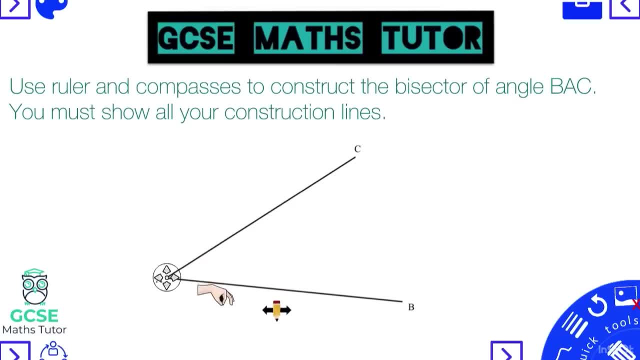 like a little arc here. So I'm just going to put that around about this sort of distance and I'm going to draw an arc in And there we go, And that starts it off. Now what you need to do is you need to take your compass and 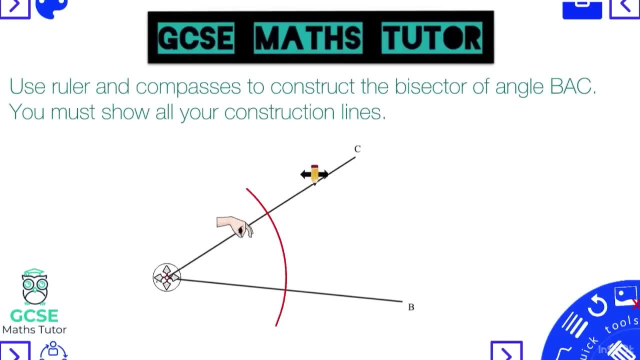 depending on how far you've gone out, you need to extend your compass a little bit further, or if you've gone already quite far out, you might want to just go a little bit closer down. here. I'm going to go a little bit further out. I'm going to draw another arc at this. 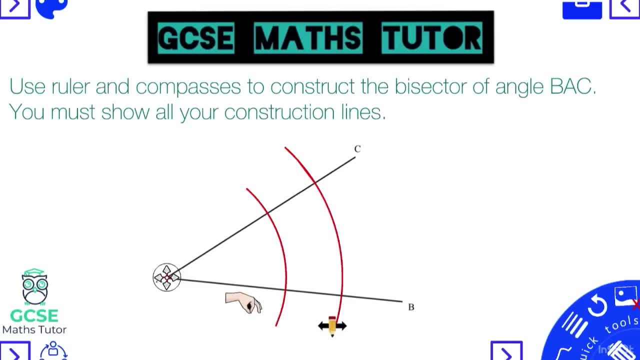 longer distance down the line. So I'm just going to go again And there we go. Now we've got our two arcs, All right, And so we are done with our compass for the moment. So we'll get rid of our compass And from here you'd need to grab your ruler. 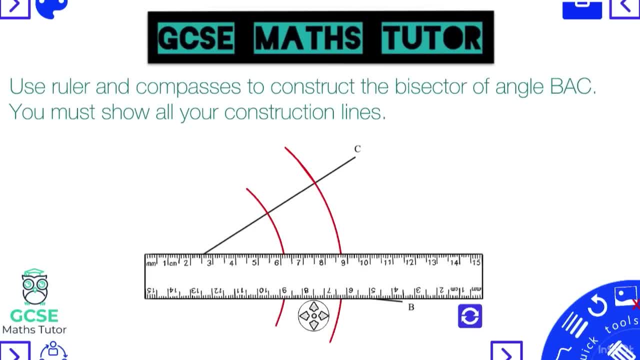 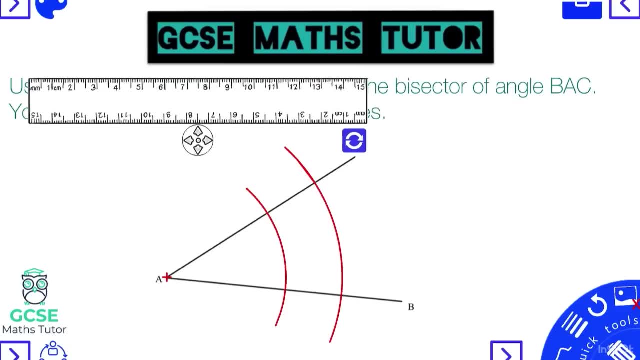 So grab your ruler. I'm going to try and use this one. I might not be able to do this very well on screen, but I'm going to try and use this ruler. What we're going to do is: we are going to connect. I'm just going to put that over there. We are going to connect. 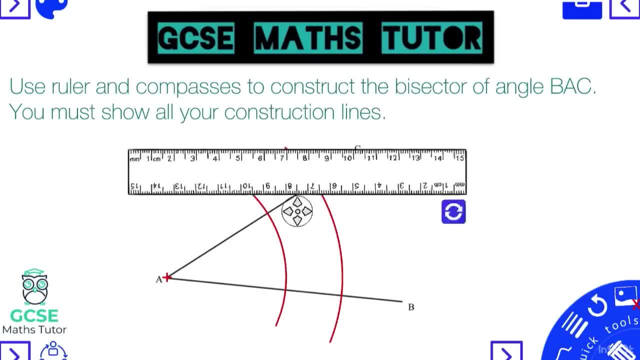 some of these points and do what I call a little crisscross. So I don't think I'm going to be able to do this with the ruler, but I'm going to show you what I kind of mean. So we're going to go between around about there. There we go, These two points just. 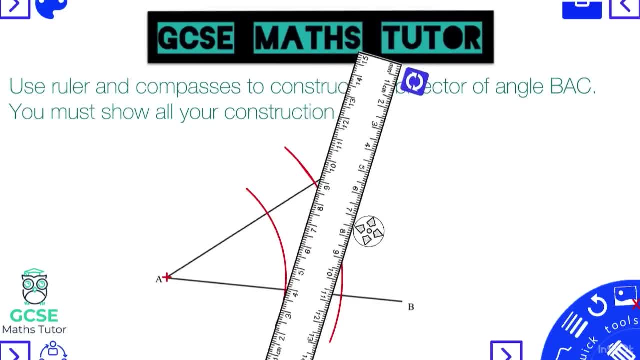 here. I'm not going to be able to get that perfect with the ruler, but we're going to go between these two points and do a little crisscross, So let's just move that out of the way Just using the pen. Let's swap colours. Let's go for blue. So from this point over here, 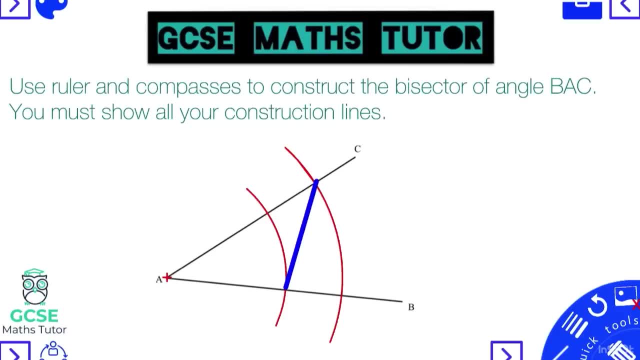 to this point. So we're going to do a little cross between the right or the bottom side, on the bottom line, to the top side, on that top arc there, And we're going to do the same with the other two. So another little crisscross from here to here. There we go, And where? 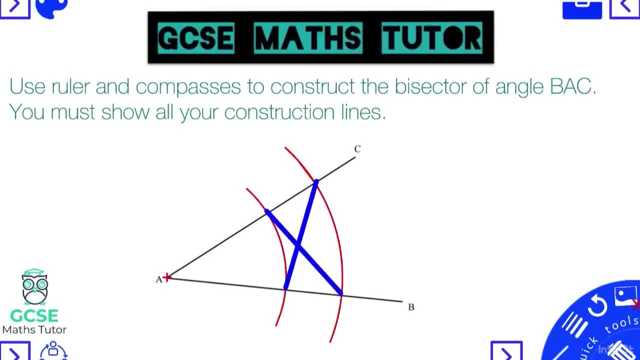 those two lines meet, which should be a lot clearer when you're doing it with a pencil on paper. That is right in the middle of this angle. So the next step is we're going to take our pencil again. We want to draw a nice straight line from point A where that little cross. 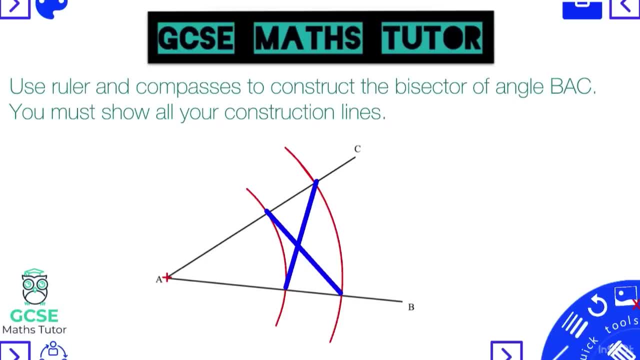 is straight through. Let's have a look and see if we can draw this straight through the middle where those two construction lines cross. There we go. I'm just going to leave that there And there we go. And for this question here, as with all these exam questions, 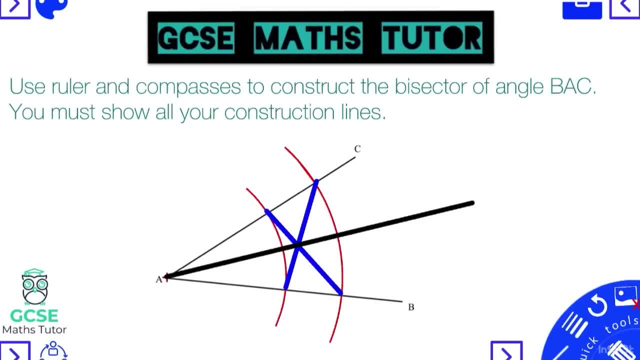 here, when you're doing loci and construction. it does say- and it says it in the final question: you must show all of your construction lines. So don't be tempted to start rubbing them out. Don't worry that it looks a little bit messy. We're wanting to see those construction. 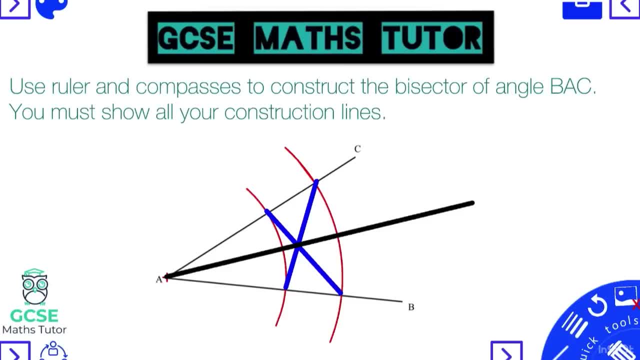 lines and seeing how you've actually bisected this angle. But there we go. That's how you bisect an angle. So you draw one arc, one slightly bigger arc, and then do your crisscross and join together through the centre, right there Now. 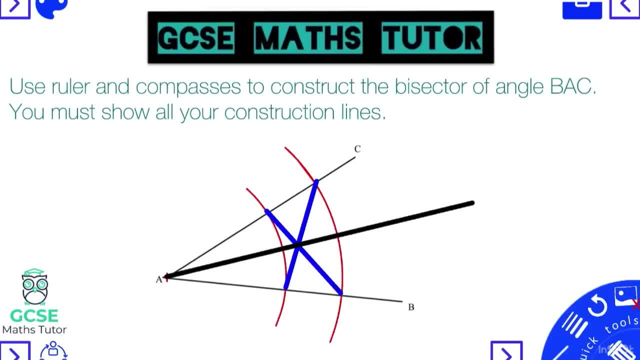 there is another way of doing this. I do think it's a little bit slower, so I'm not going to go over that method, because this is the one that I prefer. I think this is a really nice one to remember. You just do two arcs, crisscross and straight through, And there. 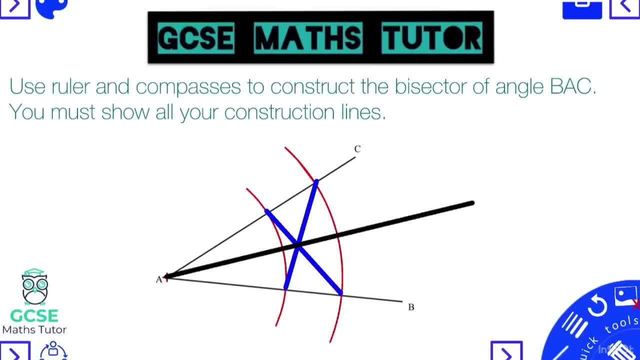 we go. That's how you construct an angle bisector. Now we're going to have a look at a perpendicular bisector to a line. There are a few different types of questions that you could have with a perpendicular bisector, So we've got three. 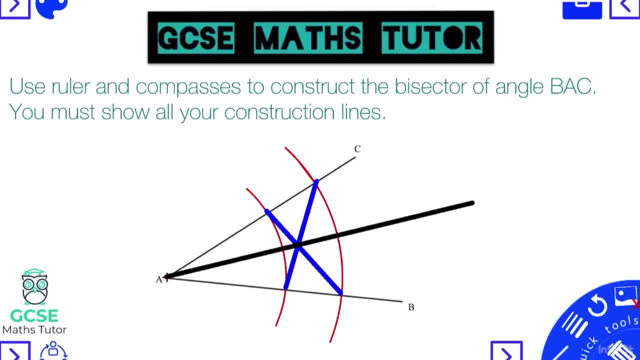 of those to have a look at, And then, on another video, we're going to have a look at some exam style questions. But there we go. That's how you construct your angle bisector. So what I would suggest is drawing a few angles on some paper, having a practice, doing a 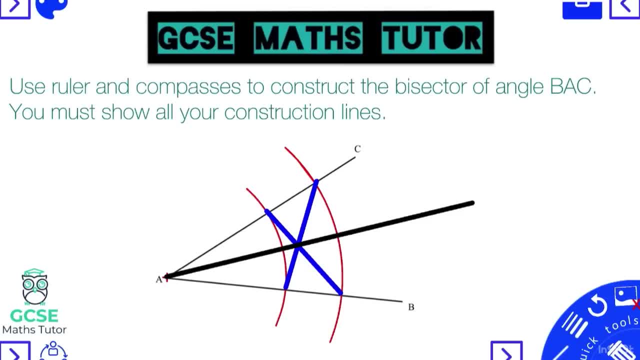 few of these And just rewind the video and rewatch that if you need to Have another go at doing that or you're not sure exactly on the method, So maybe just put it on repeat while you're doing it and hopefully that should help. 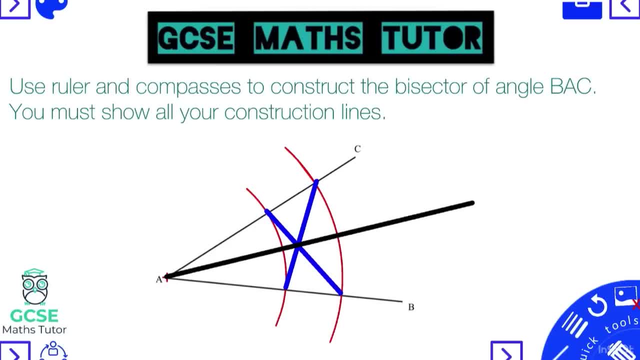 All right, let's have a look at a perpendicular bisector. Okay, here we go. So for a perpendicular bisector. again, a bisector means to cut it in half, And we're going to cut it in half in a perpendicular way, which means at a right angle. So we're. 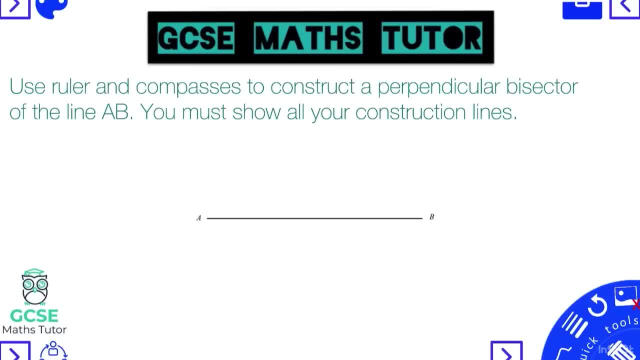 going to put a perfect right angle, a perpendicular line, through the centre of this line. So we're going to cut it in half. So, to start with this, we are going to use our ruler a little bit in this one, although you can actually get away with doing this without a ruler- But I'm just going to put 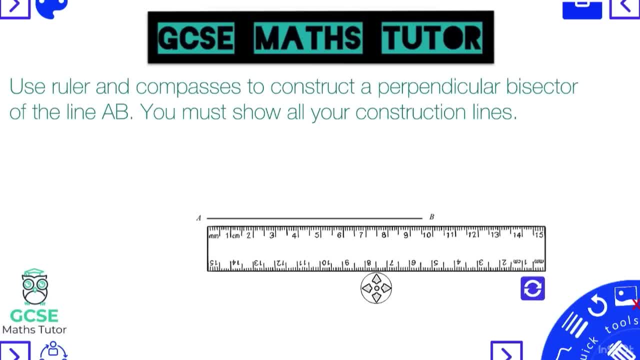 this ruler at the start of the line. I'm just going to have a little measure of it. Let's have a look. And mine comes out as 9.5 centimetres. This is going to be important when we do our perpendicular bisector here, as you're going to see, when we do these construction lines. 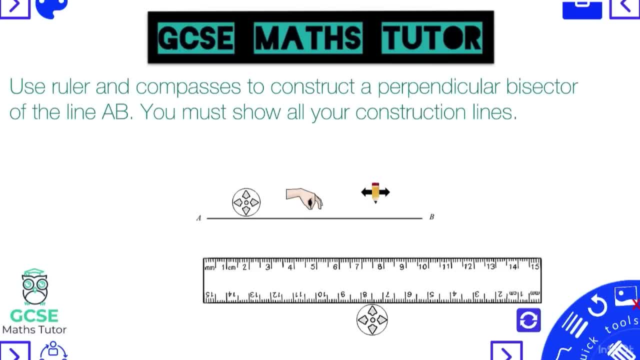 So again, grab your compass, make sure it's got your pencil in there, And here we go. So first things first. I am going to put my compass point on one of the line ends, or the ends of one of the lines. I'm going to stick it on A to start with. Now what I need to do is I need to extend. 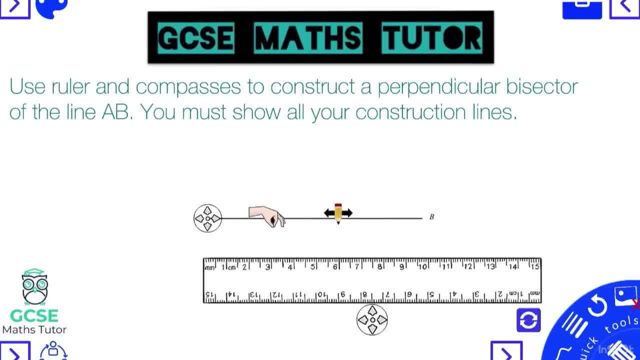 my compass past halfway down the line, So you don't really need the ruler for this. We could line it up and we could say, okay, well, it needs to go past four and three quarter centimetres. We're getting a little bit too trying to get it too perfect there, But all. 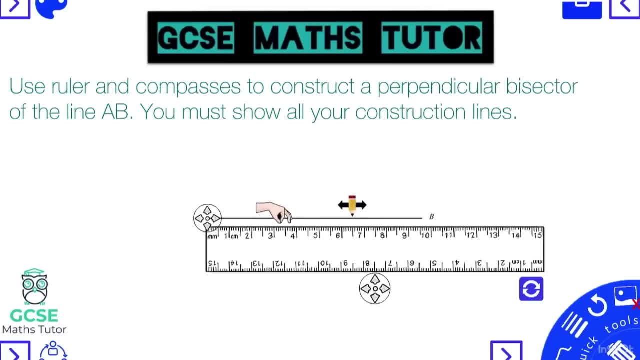 we actually need to do is go past halfway, And you can tend to do that without a ruler, So we shouldn't hopefully need it. But if I go past the centre, there we go. Now it's on six centimetres. I'm kind of done with my ruler now. I don't really need that for. 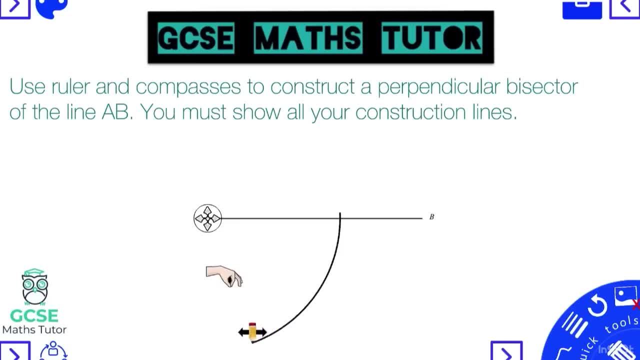 the moment. But I'm going to draw a nice big semi-circular arc. Actually, let's see maybe if we can do that in a different colour. There we go, A nice big semi-circular arc. from that point. There we go. Now, what I'm going to do is I'm not going to change the distance of the compass. 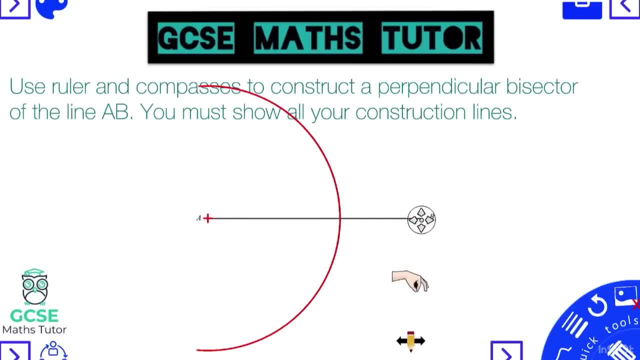 So I'm going to take the point off point A and move it over to point B, leaving the compass exactly the same length, And then I'm going to do a nice semi-circular arc the other way. There we go. We get this nice cross over here. 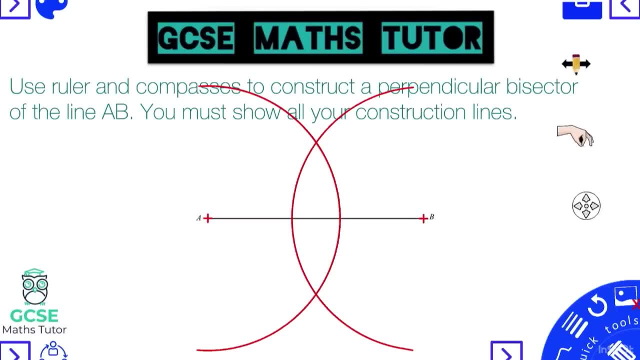 Where the two arcs meet. So let's move our compass out the way. We don't need that anymore. We've got the one at the top there where they cross over and the one down below the line where they cross over down the bottom. 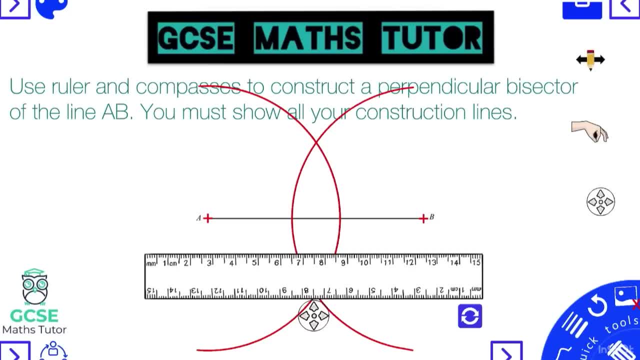 So what you need to do, grab your ruler, And I'm probably not going to be able to do this perfectly on the screen, So I'm going to do it with a straight line. I think I'm drawing all over the place, So put your ruler in between those two points. just there, There we go And join them up. 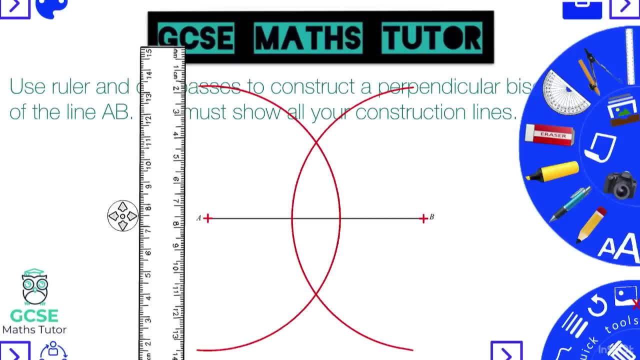 with a nice straight line. I'm not going to be able to use that. I'm going to use the ruler, perfectly. So I'm going to do this with a pencil and see how we get on here. So, straight from that point down through that one, There we go, And that is how you would. 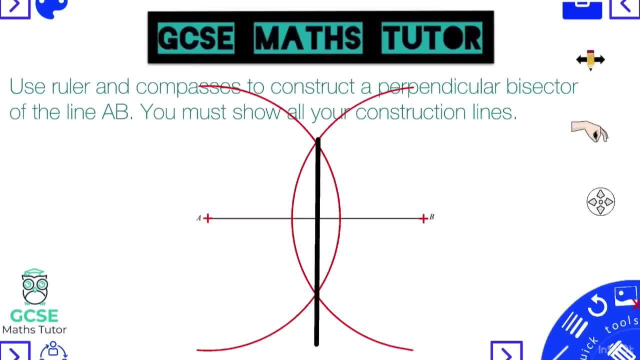 constrict your perpendicular bisector. Not perfect on the screen while I'm doing it because I'm not able to use that ruler perfectly, but that's how you constrict a perpendicular bisector. There we go, And that has cut at a nice 90 degree angle to the line straight through. 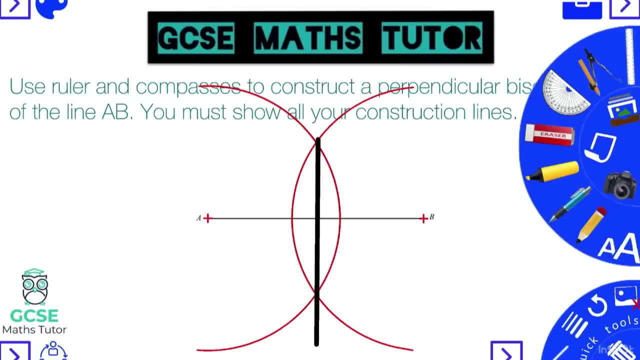 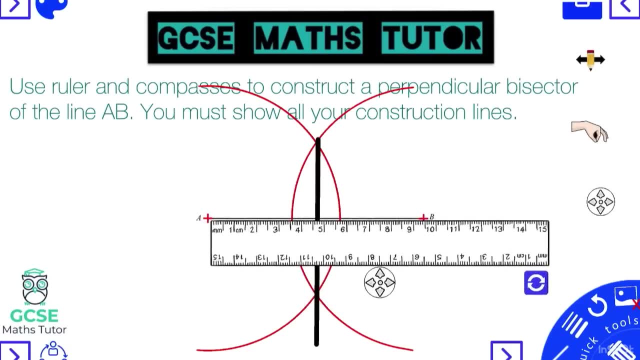 the middle. Now what you can do. you can actually grab your ruler and you can measure the line and you can just double check to make sure that it goes halfway through. It's obviously a little bit difficult to read on my screen, but there's a nice way there for you just. 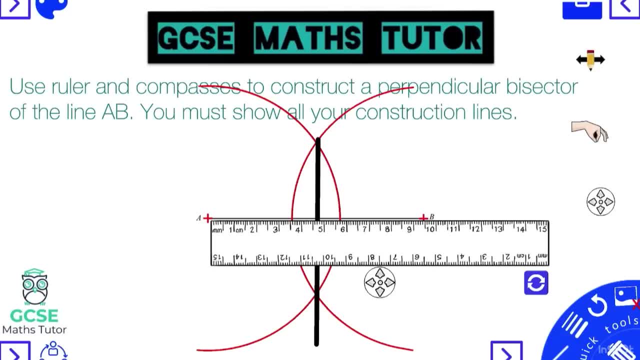 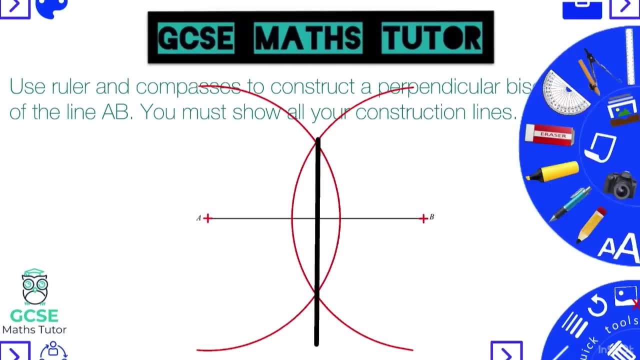 to double check and make sure it's definitely gone through halfway and therefore it's definitely a bisector You could even grab if you wanted. let's have a look, Here we go, Your protractor. You could stick it on there and you could actually measure to see that that's a 90 degree. 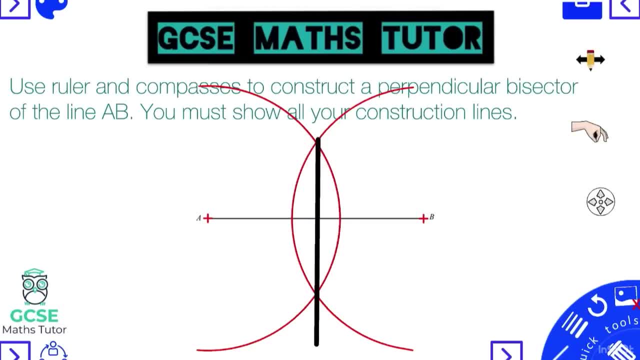 angle as well. So lots of different things that you can do to check to make sure that it's perfect, But if you follow these steps, they're always going to be pretty much perfect. Okay, So there we go. Right, We're going to have a look at another type of perpendicular. 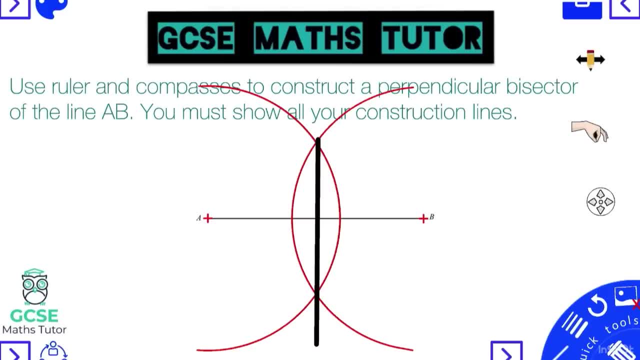 bisector, where we have to actually bisect it in a different position. Okay, Or just actually create that perpendicular line through a different position of the line, rather than smack bang in the middle. Okay, Let's have a look at that one now. Okay, Here we go. So a slightly different type of 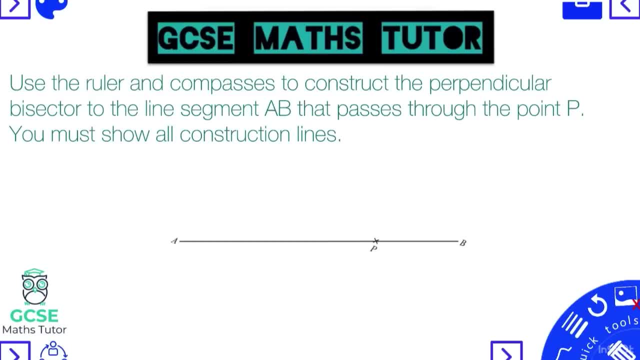 question. Now again, if you want to follow along with this, all you need to do is draw a line and put a little cross somewhere that's not in the middle to show, like my point P in my diagram. It says here: use a ruler and a compass to construct a perpendicular. 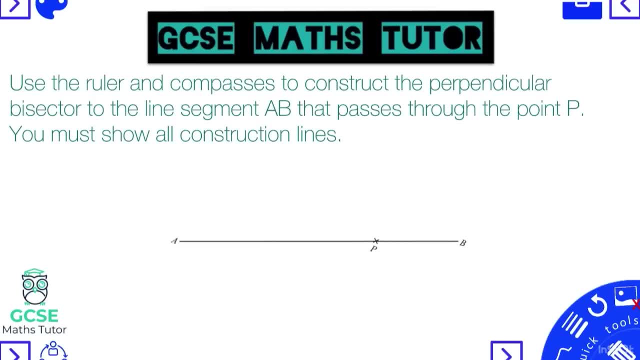 bisector to the line segment which is shown below AB, and it passes through point P And you must again show all your construction lines. So, just like that first one, we're not going to get rid of any of these construction lines. Now, if I want to cut it through point P, I've got to be a little bit more careful here, because 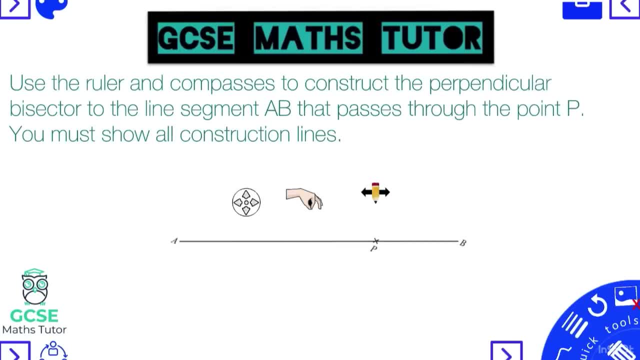 if I was to get my compass, there we go. and I was to put it on point A, go past halfway, I'd end up making a bisector through the middle of this line. Now I don't want to do that. I want my bisector to go perfectly through the point P. So what? 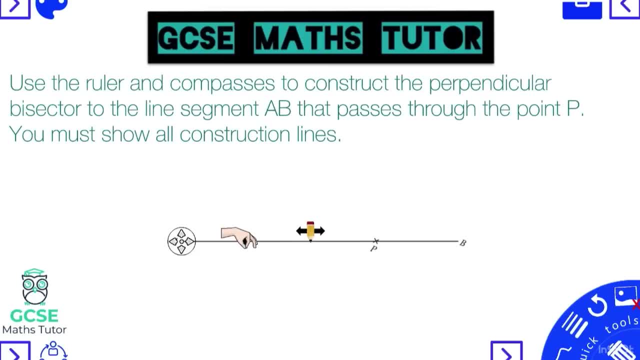 I want is I actually want that point P to be in the centre of my line, that I'm going to bisect, And to do that I need to get my compass and I need to put it on point P. I'm just going to spin a circle around the line like this, so that P is in the centre of it. 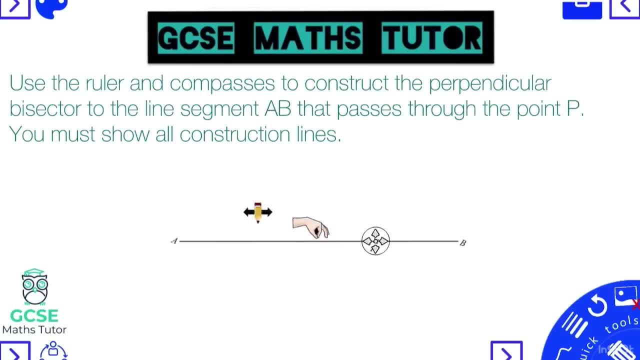 So you can put your compass as well to the close line. I don't want to do it over here because that's going to make a big circle. I'm not going to be able to actually find the line over here, But near enough, on the end of the line, just there, I'm going to spin that round There. 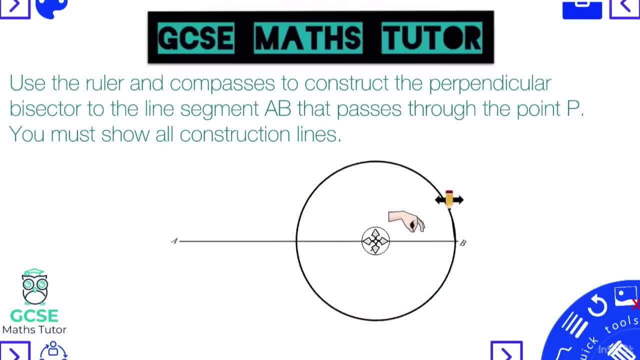 we go, And that's going to be the new line I am going to actually bisect. Now you can actually get rid of a little bit of this, just to make it a little bit easier, because you can have a lot of construction lines everywhere. The important part was actually: 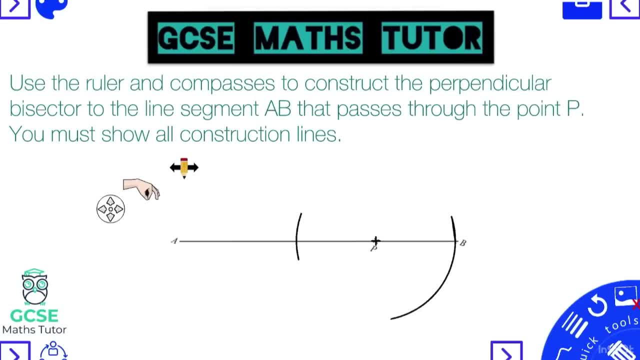 splitting the line. There we go. So I could have just put those little arcs in just there And that's going to perfectly split that line in half. So now I have my new line And if I do a perpendicular bisector of this smaller line, that's going to actually cut straight through. 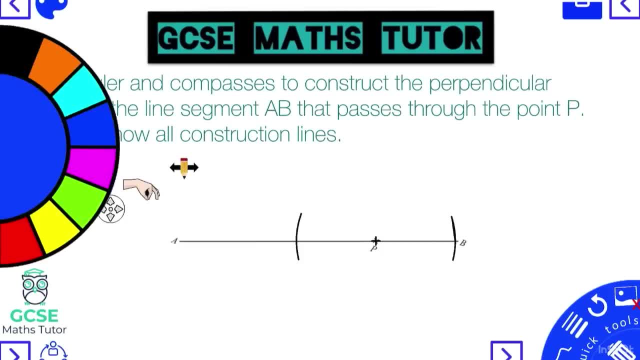 P. hopefully, okay, Hopefully, because obviously it's a little bit difficult to get these perfectly accurate, but we're going to do our absolute best on it. So, again, following the same sort of process, we'll get our sharp end of the compass stick. 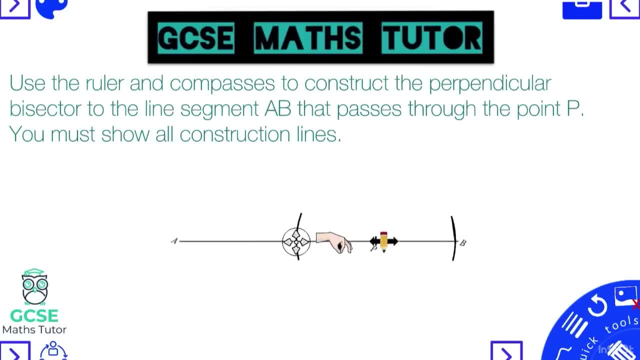 it on the end of our new line. And again, this is actually marked out halfway now, so I just want to go just past that. You don't have to go too far past here. I'll go just here. And again, that's definitely not going to be the right size. Okay, let's swap to. 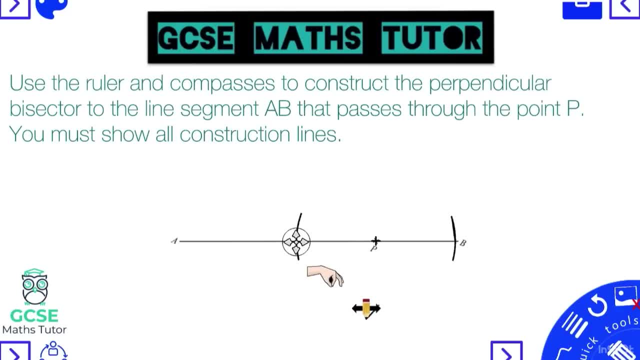 a pencil. I think I was still on the rubber there. There we go. So let's do a nice arc around And again, let's do this in red actually, just to make sure we can see that that is our construction line. There we go. Again, do not change the size of the compass Move. 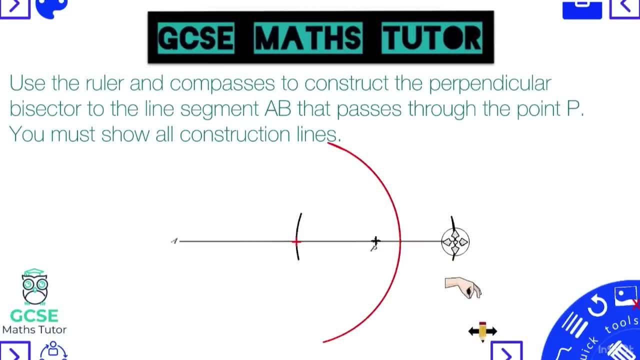 it over to point B. There we go, And we want to draw another arc all the way around. There we go, And again you can see we've got those same construction lines that we had before on our perpendicular bisector. Now again, you just want to get your ruler. 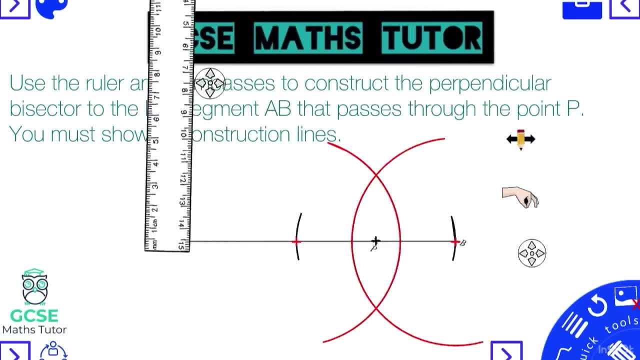 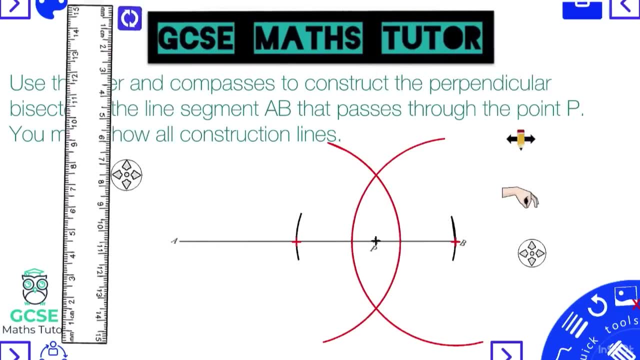 You want to make sure it's nice and vertical and it's going perfectly through these two lines and just join those up Again. I'm going to try and join those up to the side and see if I can get these perfect. almost There we go. 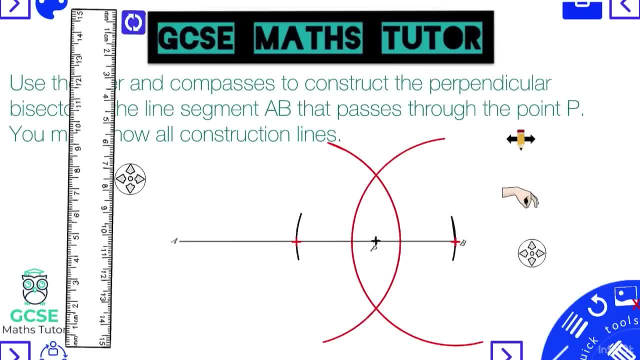 Not a straight line, though, so let's do that again. Oh, it's going to be difficult for me to get this perfect. There we go. That's probably about as close to perfect as I can get doing it on the screen here. 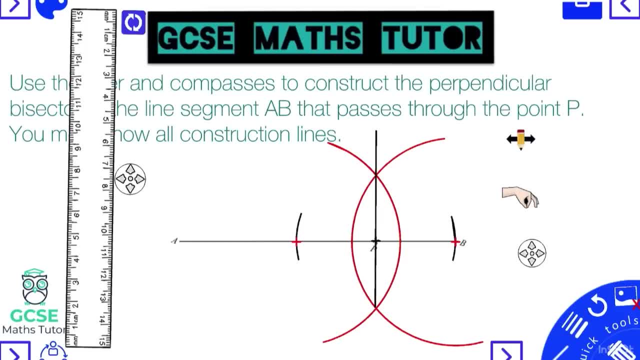 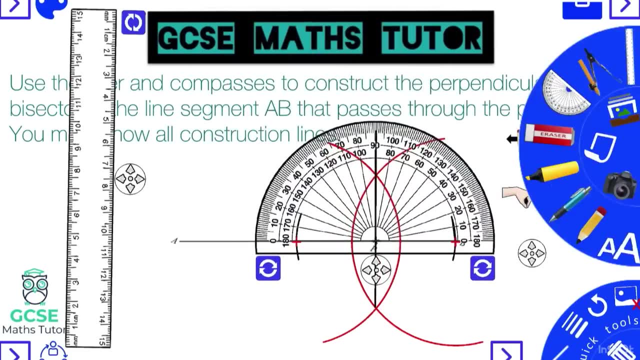 There we go. That is pretty much perfectly going through P. there Again, you could get your protractor. You could measure that out. see if it's at a 90 degree angle. Mine is, so I'm quite happy with that. 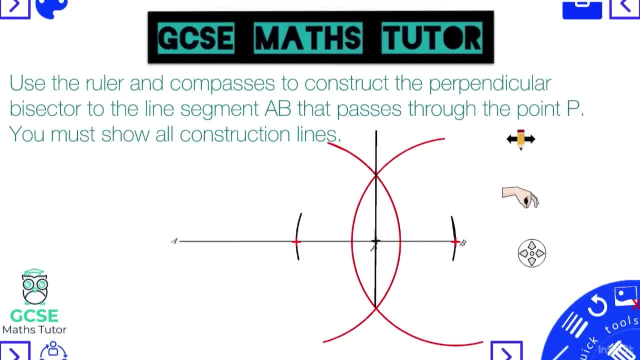 There you go. That is how you would construct a perpendicular bisector when it is going through a different point to the actual center of the line segment that you're given. I've got one more for us to have a look at and that is going to be where the point that 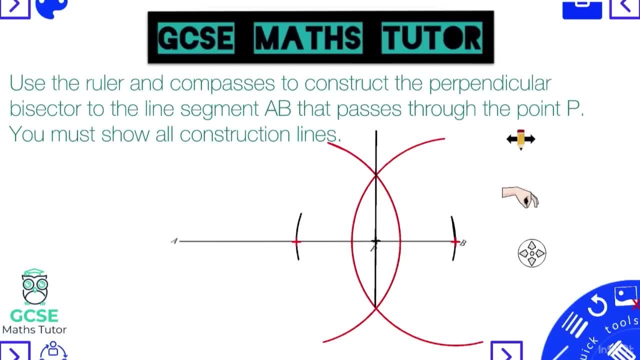 it wants to go through is actually not actually on the line at all. It's actually above the line. It's actually above or below the line, which is the one that people tend to struggle with the most. We'll have a look at that one, and that's going to be our last one. 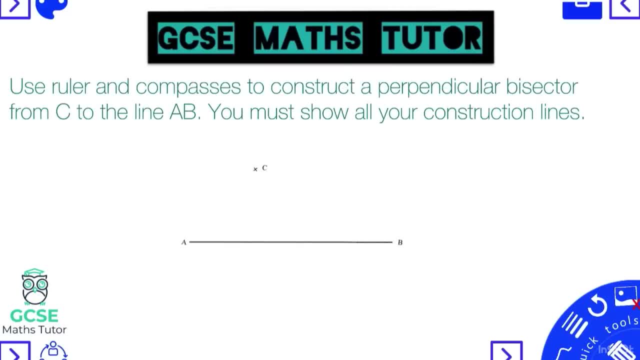 Let's have a look at that now For our last question. here we go. It says: use a ruler and a compass to construct a perpendicular bisector from C, which you can see on the diagram. there We've got that little cross hovering above the line to the line AB. 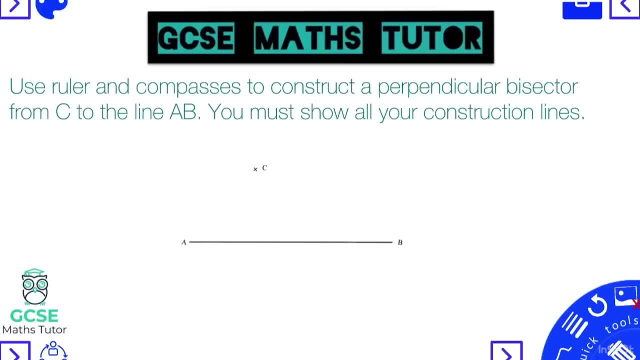 Again. you must show all your construction lines Again. what we actually want is we want that point C to be halfway between our line. Unfortunately, you can already see it: It's slightly on the left. We want to do a similar process to what we just did on the last question, just to make. 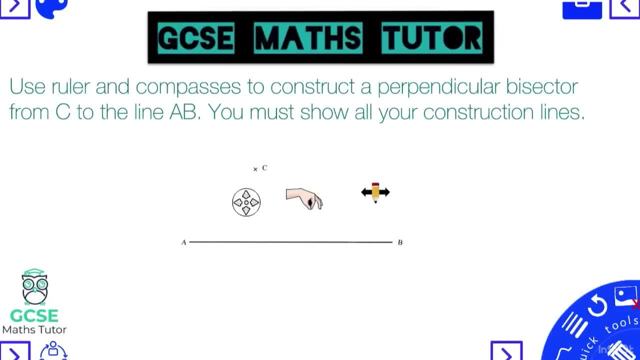 sure that C is in the middle. The way to do this: grab your compass. We're going to just make this a little bit shorter for now. We're going to put the sharp end on C again. There we go, We're going to swing an arc that just touches. 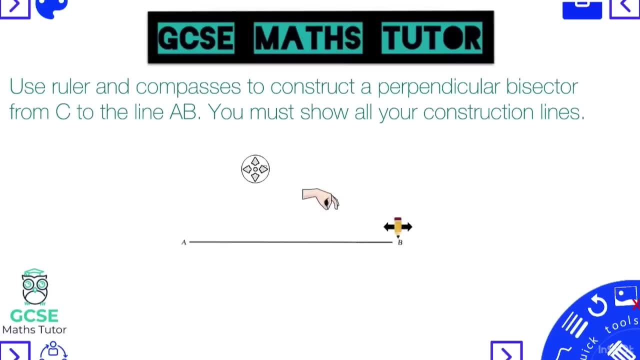 Again, we want it to just maybe touch one end of this line. We don't want to go over to B because that's going to go beyond line A. We'll put our pencil on point A around about there, We'll swing a nice little arc and that should cut the line, as you can see, into a slightly. 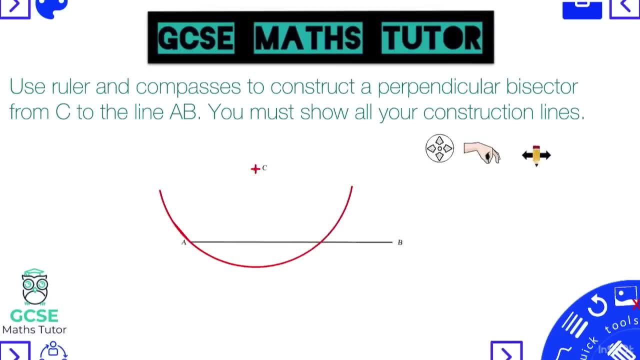 smaller line. Now, if I move my compass out of the way again, we only needed some of the construction lines here. That was really just the points at which it crosses over the line, so I could get rid of this, just to make it a little bit tidier. 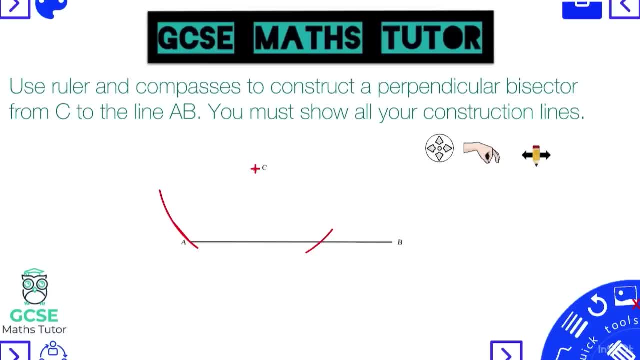 Remember, we don't want to get rid of our construction lines, but they are the construction lines there that we actually need, the ones that just cut that line down a little bit. There we go. We've actually cut the line down Again. the rest of the process is going to be the same. 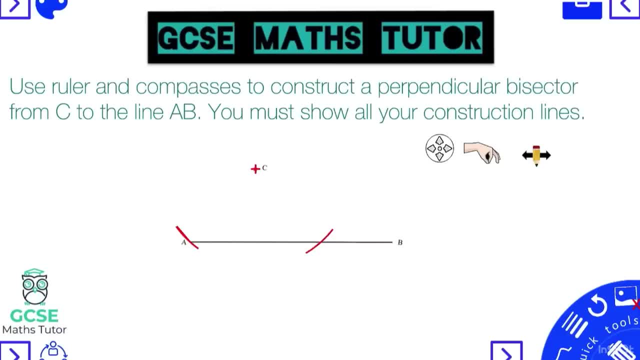 I'm going to go over to point A. I'm going to go over to point B. I'm going to go over to point C. What I want to do from here is use those little red lines to construct my perpendicular bisector. Again, if we're nice and accurate, it should perfectly go through C. Let's try it out. 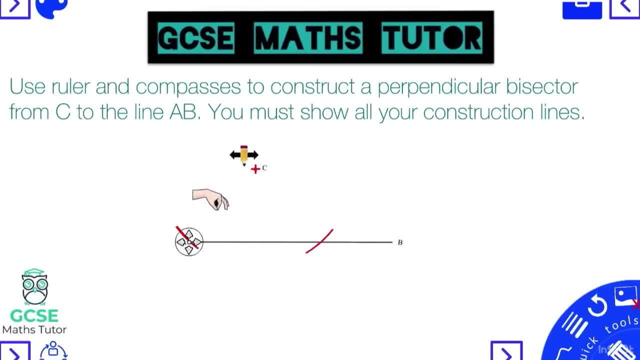 Extend your compass a little bit. We're going to go just past halfway. Again, that's going to swing up. That's probably going to go straight through C. if I go there, That's not a problem at all. Let's construct There we go.